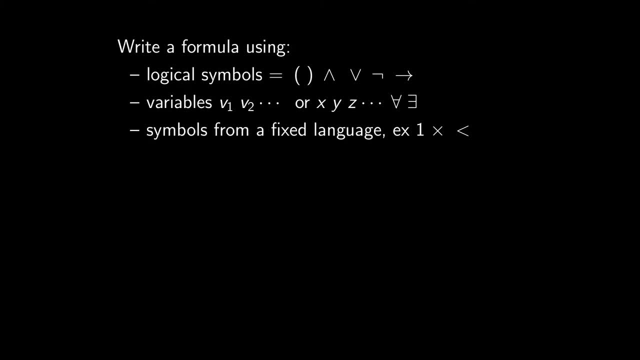 coming from a language that can change depending on what you want to express. You can have constant symbols, such as 1 or 0, function symbols such as plus times exponential, and relation symbols such as being smaller, being divisible by or any other stuff. Okay, now write a formula. 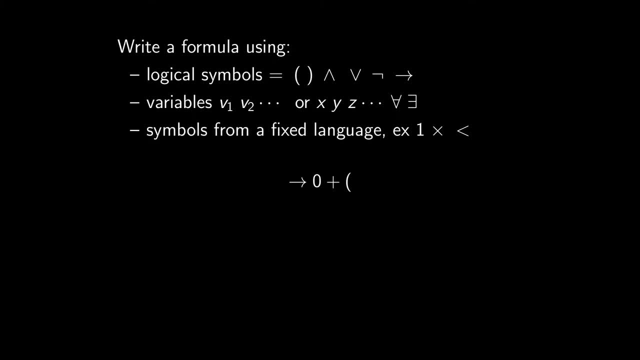 Right. well, I didn't specify the rules, but I think we can pretty much all agree that this is not a formula. This, however, is a formula, and so is this Really. if it makes sense, it's a formula. If it doesn't, it's garbage. Now, we can take a bunch of actions, put them. 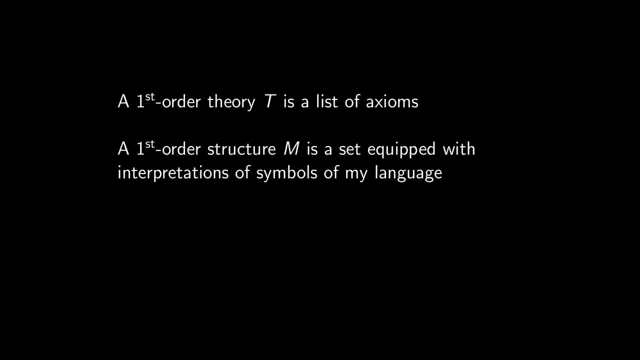 together and call it a theory. Then we can take a set and equip it with interpretation for the language and call that a structure. And if we have a structure for which all actions in the theory are true, we call it a model and rewrite it with this funny little symbol. 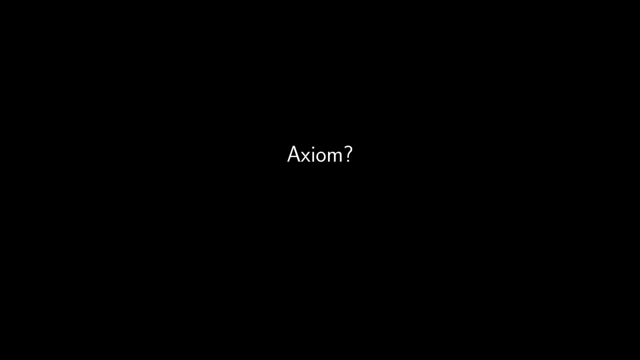 Okay, now I know what you're gonna say. You didn't define what actions are. Well, okay, let me do it. An action is a formula in which every variable is quantified. Okay, but what about the interpretation in a set of symbols of the language? Well, it just means: for constant symbols, you have a. 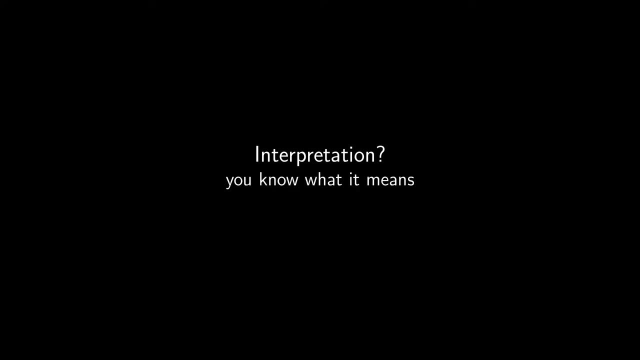 corresponding element in your structure and for function symbols you have a function, etc. It's very natural, really. But what about truth? What does it even mean for a bunch of symbols to be true in an abstract mathematical object? Well, this is also quite intuitive, Like. 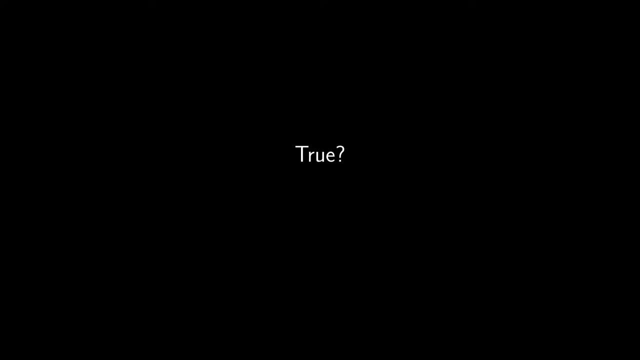 the formula there exists x such that x, square, equals minus one is true. there exists x such that x, square, equals minus one. you know, it's just what it's supposed to be. we don't have time, And I didn't even say what first order means. So, in short, 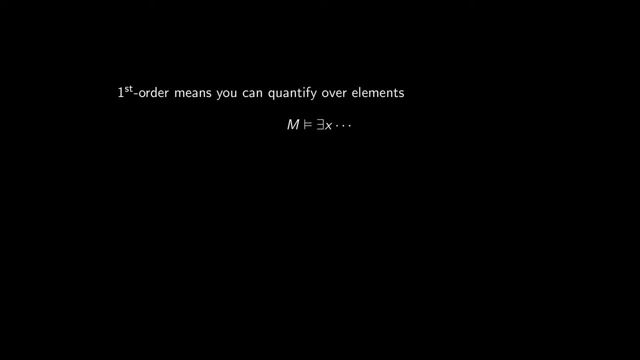 it means you can quantify only over elements. So this means there is an element x in M, such that something. Second order means in some sense you can quantify over subsets. So for example, all subgroups of R are either dense or discrete. is a statement in second order. 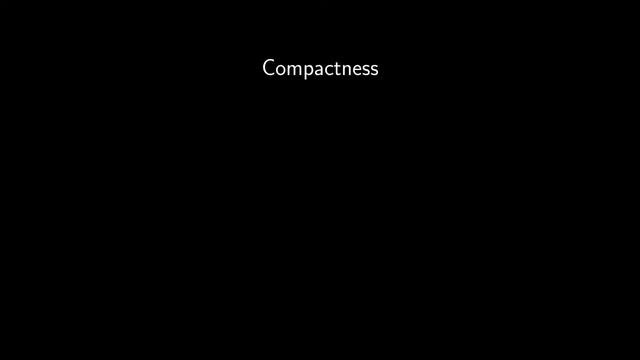 but not in first order. Get it Cool, Because now we can move on to compactness. Compactness is the final smash of model theory And it's the main reason why we only do first order, really, because in second order it doesn't really work. It says: 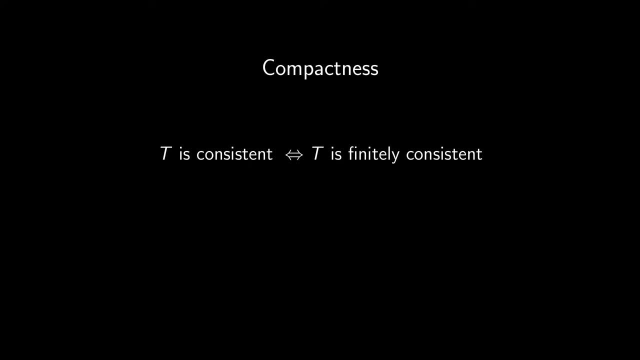 a first order theory is consistent if, and only if, it is finitely consistent. Okay, so you take a finite number of formulas from T. you prove they are consistent by finding, or, more often, constructing, a model of all these formulas at once, And provided you can do that, 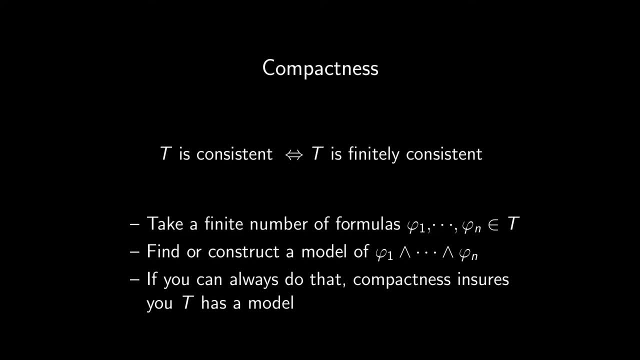 collections of formula. Well, compactness guarantees a model of the full theory. That's nice, isn't it? You don't need to check that the whole theory is consistent. you just have to prove that any finite sub theory is consistent. Well, okay, let me tell you: this is much more powerful. 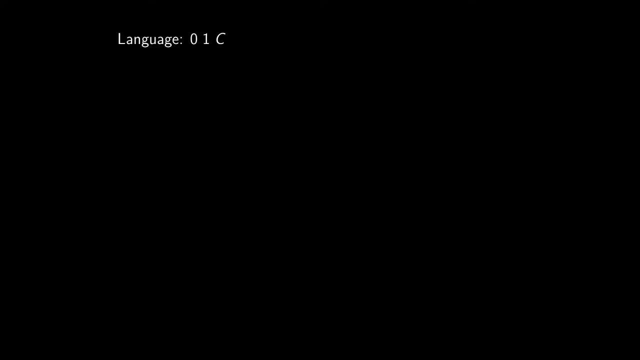 than it looks. Let me give you an example. First, we need to specify the language. The language has three constants: zero, one and C. It has three functions- plus, minus and times. And it has a relation symbol. Consider the following formula: phi n, which states that n is: 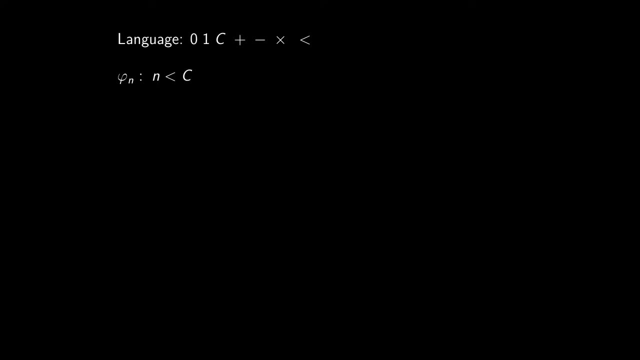 smaller than c. Okay, so n is not technically a symbol of our language, but when I say n, I actually means one plus one plus one n times, which is something you can write in first order with the symbols of this language. Now, for any n, there is a model of the theory of r. 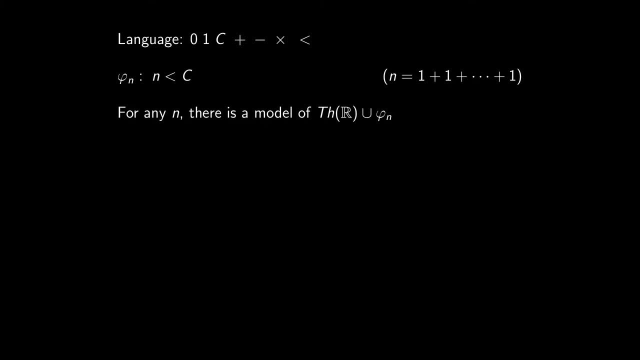 that is the list of all formulas true in r and phi n. Just take r and interpret the symbol c as n plus one. Now, because of compactness, we are guaranteed that there is a model r, star of the theory of r, and all phi n's for all n. Well then, in this model, c must be bigger than any integer and 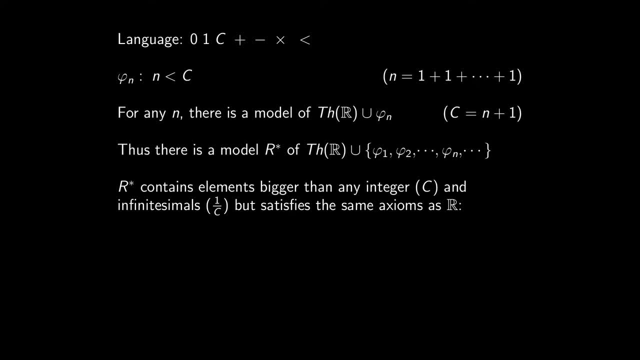 1 over c is infinitesimal, that is, it is bigger than zero, but smaller than any real number. Nonetheless, despite the existence of such weird elements, this model satisfies the same actions as r, such as any positive element as a square root or. 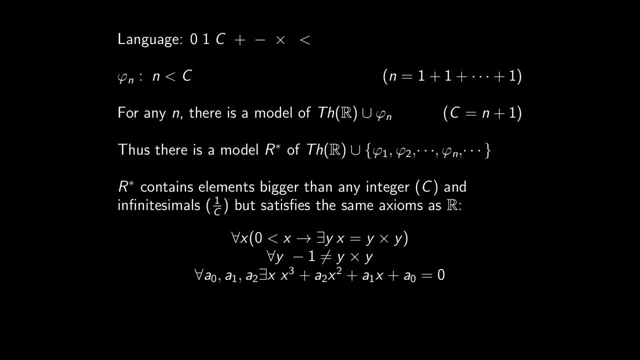 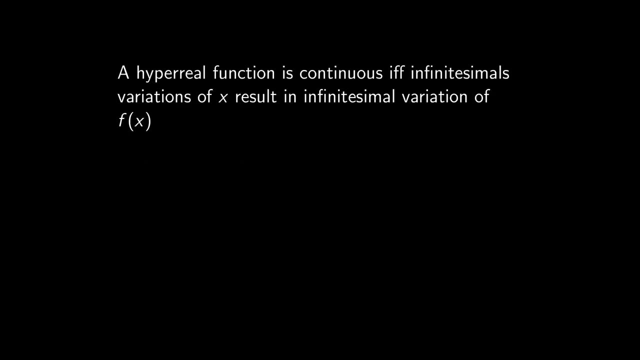 minus one has no square root or any degree. three polynomial has a root. This is what we call a hyperreal field. Once you have infinitesimals, a lot of things become so easy to state. like continuity: A hyperreal function is continuous. 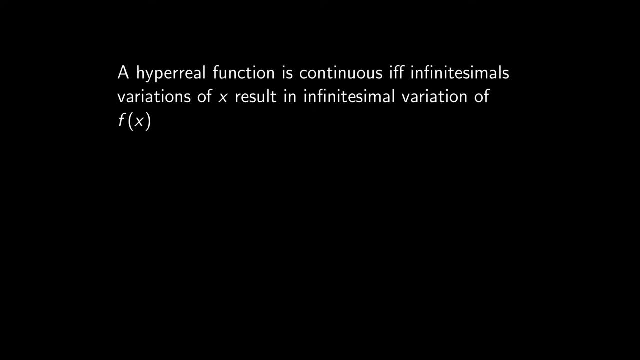 if, and only if, infinitesimal variation of x results in infinitesimal variations of f of x. How clean is that? There is no epsilon and delta getting arbitrarily small, just take infinitesimals. Much easier, much cleaner. and, may I say, this is how Leibniz himself talked about continuity. 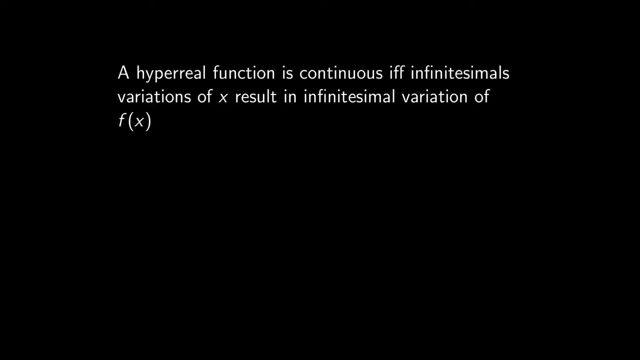 with infinitesimals. But modern theory had not been invented yet and Leibniz couldn't make rigorous the idea of infinitesimal variations. So Weierstrass, among others, came up with this epsilon-delta notation to make it more rigorous The epsilon-delta statement of limits and 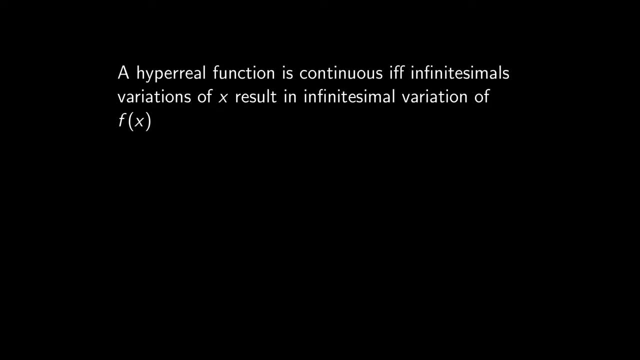 continuity and derivatives is the same as the one we saw in the previous example. So if we have special variables like real and absolute windows, the absolute and the absolute and the integral, the integral and the integral of the whole, In the end it is just a question of what are the real and the infinite cos. 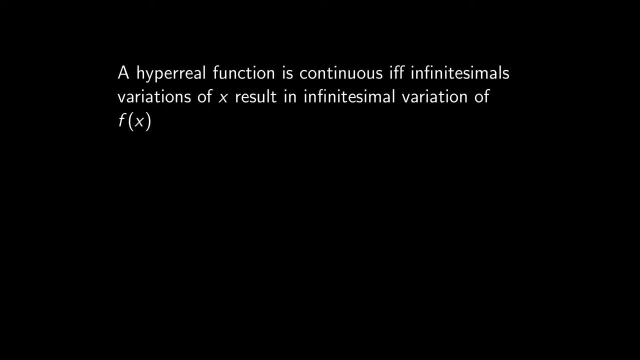 To me, the real and the infinite cos is equivalent to this kind of statement with infinitesimals. I find them much cleaner and much more intuitive. So, thanks to Robinson and other model theorists of the 20th century, we have a new way to talk about continuity. This is called nonstandard. 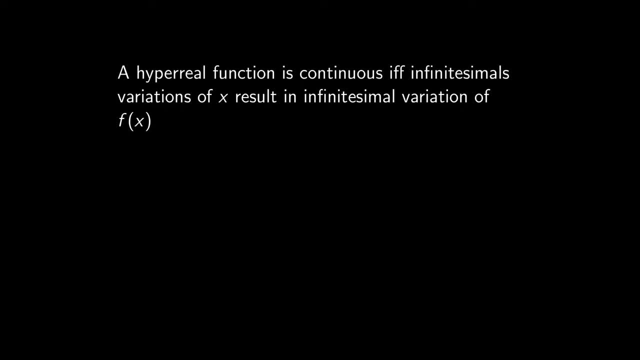 analysis. You can look more into it. there is some link in the description. Just to reassure you, you can go from a real function to hyperreal function quite easily by doing compactness and since the continuity of a real function is important, you can go from a 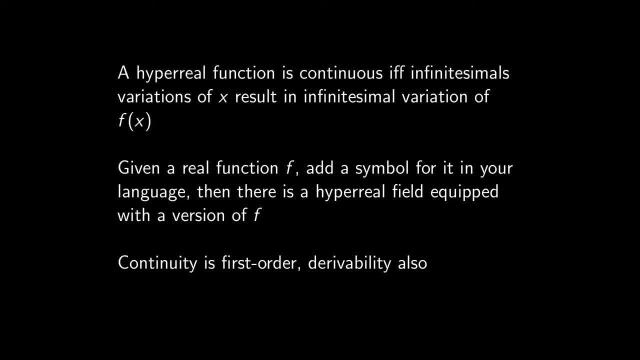 hyperreal function to a hyperreal function quite easily by doing. compactness, Derivability, limits etc are all first-order. Anything you can prove in a hyperreal field is also true in R. All the suffering you went through when learning limits, Cauchy sequences. 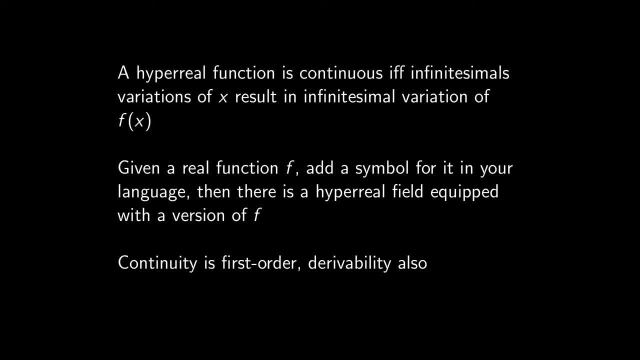 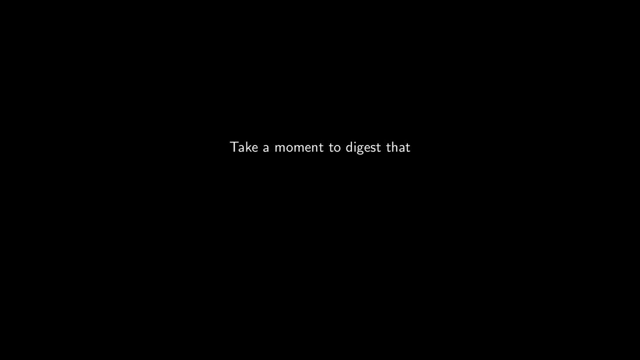 derivations could have been avoided had we known earlier about compactness. Hey, quick question: Is this function subjective? OK, well, let's see. I'm taking three coordinates in C and I want to find a common root for three polynomials. 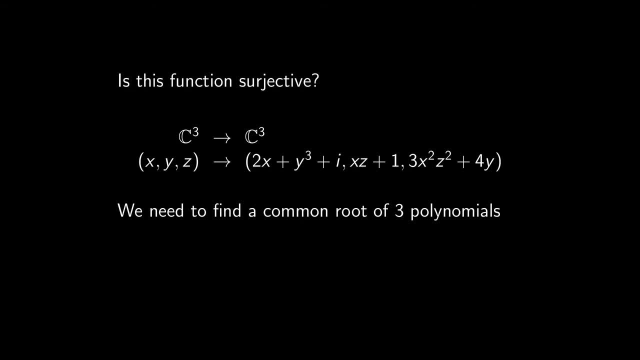 Hmm, Can you do it? Because I sure can't. We'll try to find another way. Let's have a butcher at finite fields. The simplest ones are f, which are just the integers modulo p, But there are many others, so let's try to study them. First of all, any finite field must roll back. 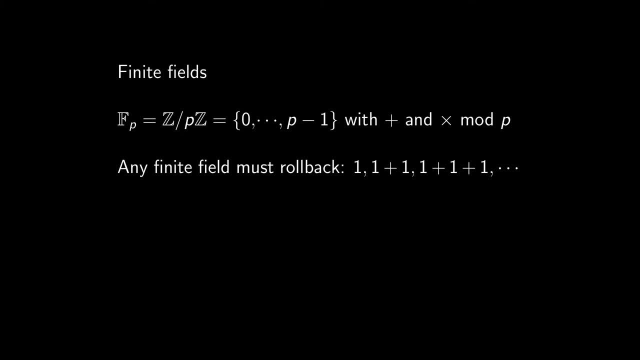 If you add one to itself enough times, you can get the same result. You must roll back because you cannot take infinitely many values, because you are finite, So at some point they will be equal, and then by subtracting one side to the other. 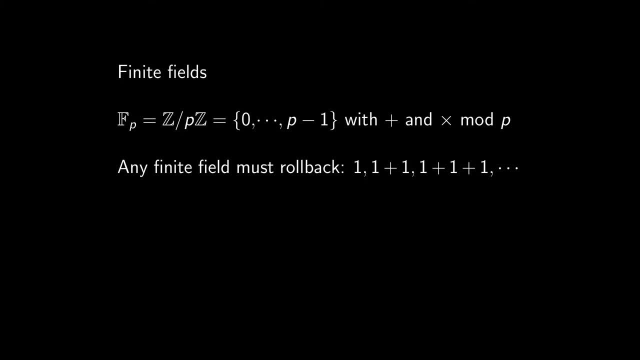 you can say that adding one to itself will result to zero at some point, And you can convince yourself that this must happen for a prime number, p, Which means that in any finite field there is a p, such that p equals zero. 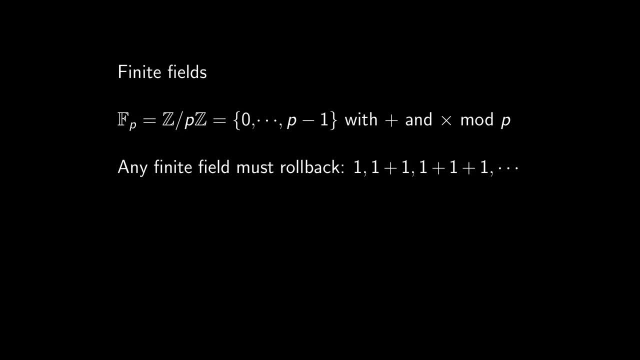 Which means that a finite field must contain f. Actually, it means that it must contain p to the n elements- And with a bit of algebra you can convince yourself that it's much harder than there is a unique field of size: p to the n, for each n and for each p. 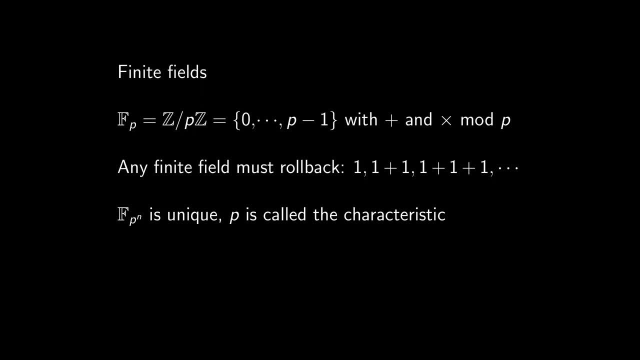 p is called the characteristic of the field, and again it is the prime number, such that p equals zero. Now if you take the union of all finite fields of characteristic p, you obtain an algebraically closed field of characteristic p. It means any polynomial in f has a root and p equals zero. 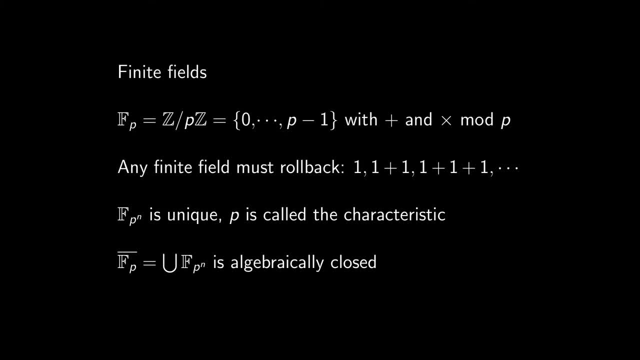 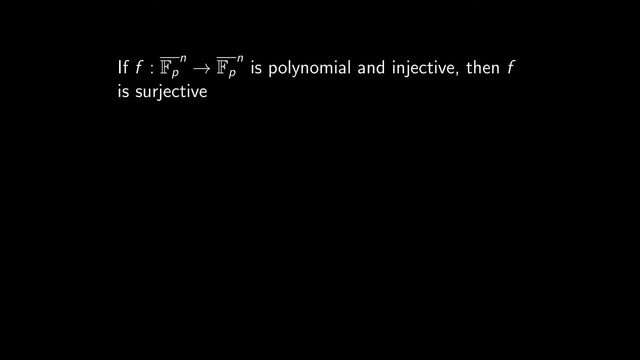 This field, f has many interesting properties, but we'll focus on one of them. If a function from f to the n, to itself is polynomial, meaning each coordinate is a polynomial on n variables and also injective, then it is surjective. 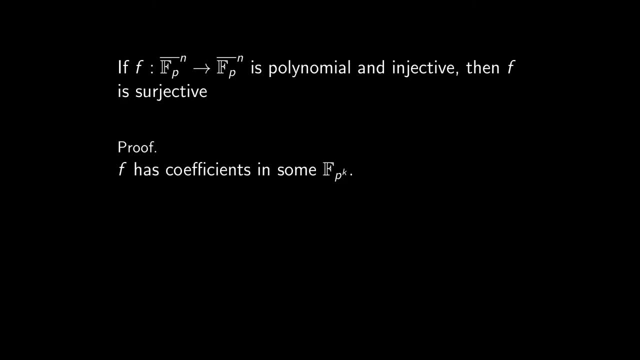 And we'll prove it. First of all, f has coefficients in f, which is the union of all f. so actually f has coefficients in some f. Now the restriction of f to f, to the n provided l is bigger than k. 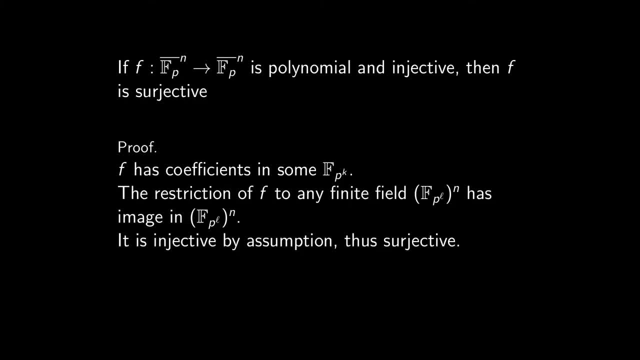 has a mate in f to the n. f is injective by assumption and since we restricted it to a finite set, it must be surjective from f to the n to itself. Now, if you take any point in f to the n, 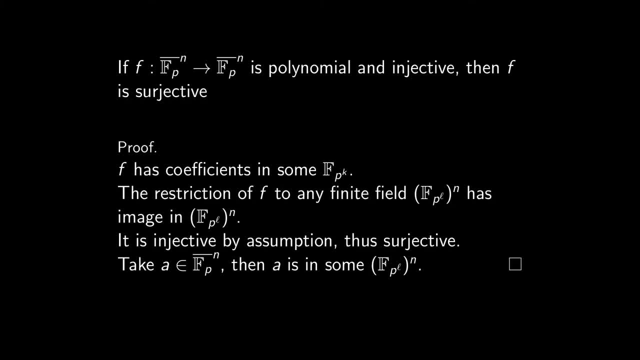 it must lie in some f to the n, so we know f will reach it at some point. Feel free to take a break and review this step of the proof for yourself. Can you see how it goes, And can you see how much of this proof relies on the fact? 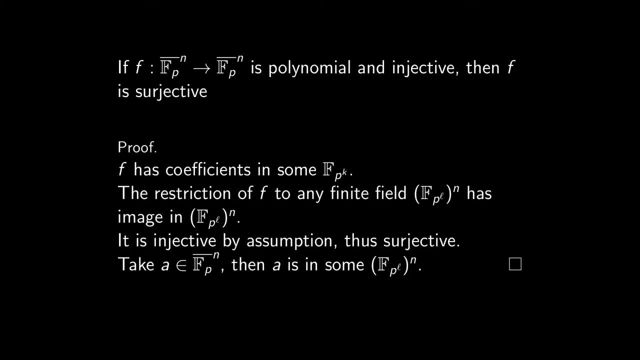 that f is a union of finite fields. This kind of proof wouldn't work for any other algebraically closed field, let alone C. But I would really like to prove it in C. Could I, for example, cheat by using something called the compactness theorem? 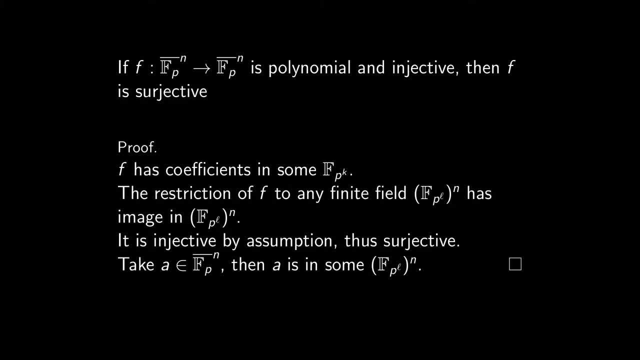 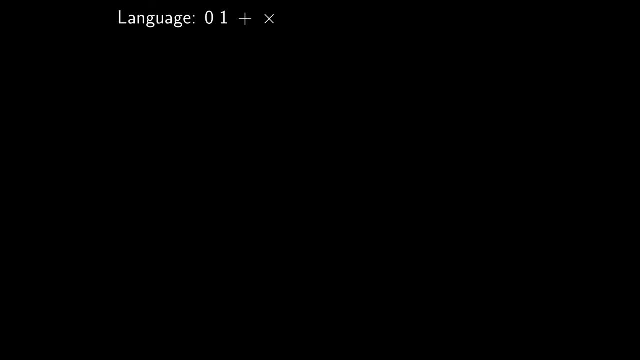 on which I'm making a video right now, and since I'm writing the script, I guess it makes sense for me to use the compactness theorem. Well, to use compactness, we first need to state the theorem in first order. Here's my language. 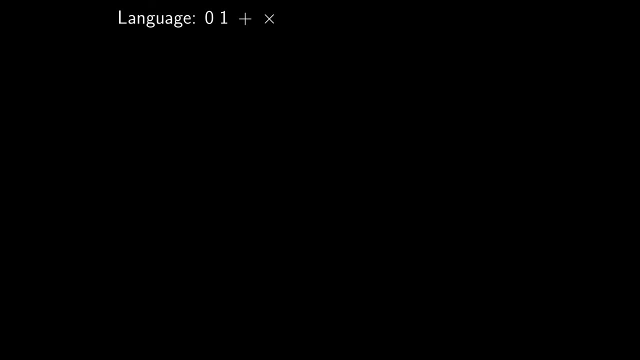 It contains 0,, 1, plus and times. In this language I can write a formula saying a polynomial function f on n, coordinates of degree less than d and with coefficients a is injective. We just write for all y and z. 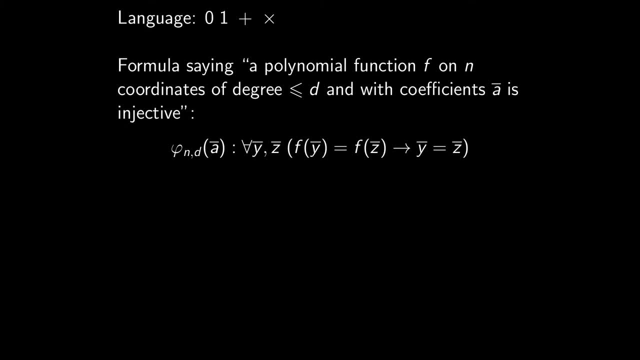 f of y equals f of z implies y equals z. Of course f is not in my language, but polynoms can be written with plus and times. I just need coefficients, which are here put in non-quantified variables of my formula. 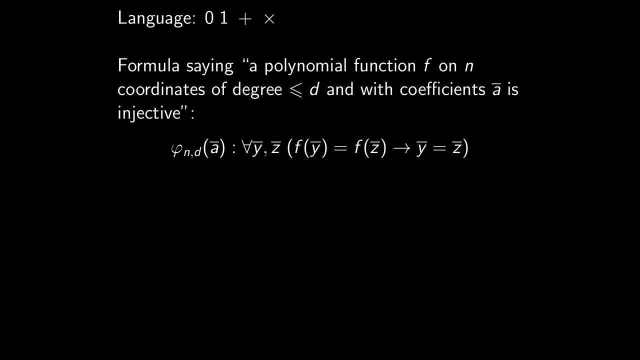 And I specify n and d to make sure my formula is not infinitely long. If you don't really believe that I can write things like that, you can check in the description for my main source, where the formula is written more precisely. Similarly, I can talk about surjectivity. 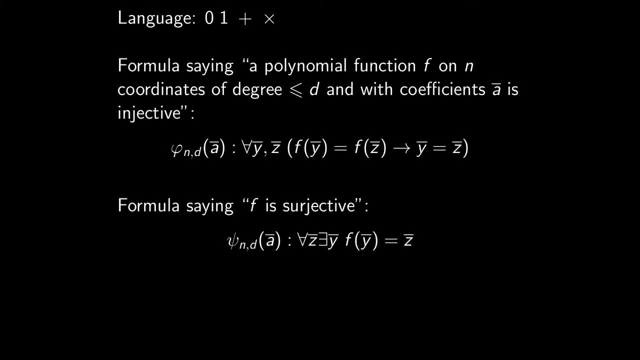 with the same caveats as before. And finally, I can just write: injective implies surjective. I'll just name this formula delta n- d, And note that delta has only quantified variables. so it's an axiom And I can now write a theory: t. 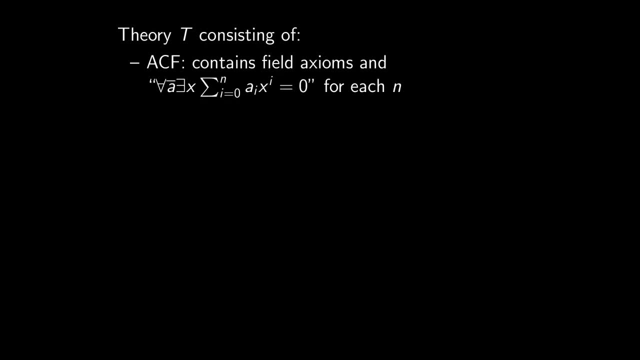 consisting of ACF, which is the theory of algebraically closed fields, So it contains field axioms such as: for all x, x plus 0 equals x, etc. And it also contains an axiom saying that any polynomial of degree n has a root. 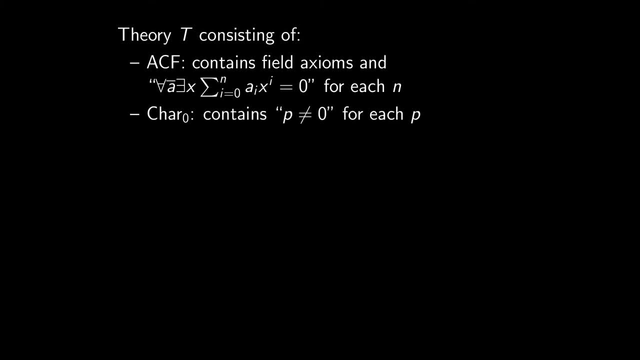 t also contains char 0. char 0 says the field is of characteristic 0,, like q, r or c. It means you never roll back. You never have p equals 0 for any p. So that's what char 0 contains. 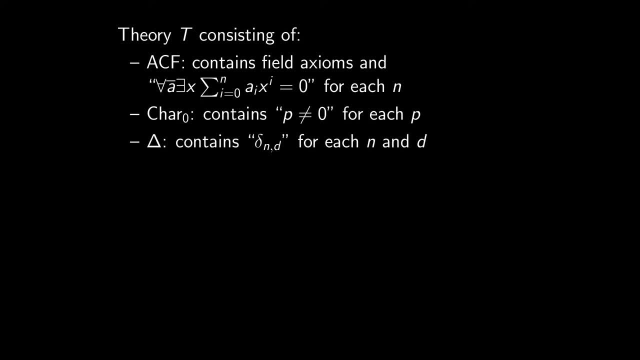 And finally, t contains delta, which is just all deltas, n, d, for all values of n and d. So t is saying that any polynomial function which is injective is also surjective. We want to use compactness. We take a finite subtheory s of t. 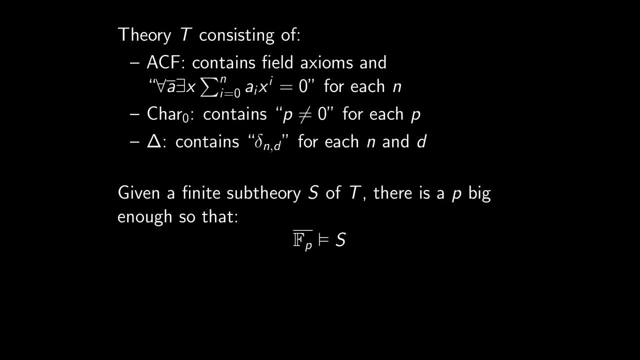 and we find a model for it, Since it only contains finitely many formulas. it only says p is not 0 for finitely many p. So I can find a prime- not in this list- and fp bar will be a model of s. 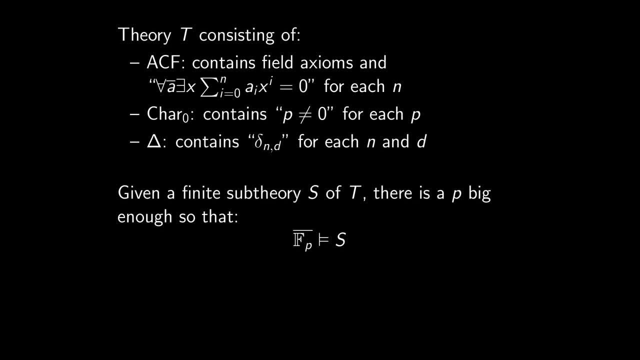 It is algebraically closed. so it checks any subtheory of ACF. It checks delta, as proven before. so it also checks any subtheory of delta And since I chose p, which doesn't appear in the finite list of formulas presenting this subtheory, 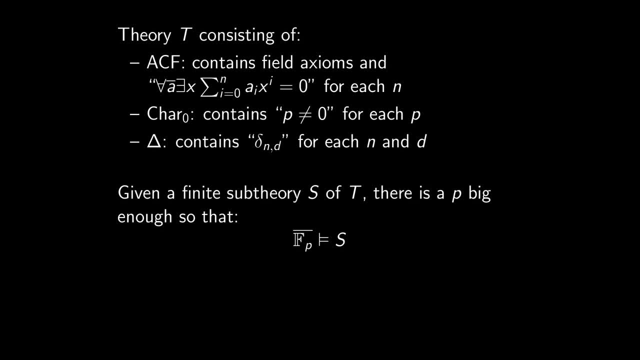 it also checks the subtheory of char 0. Therefore, for any finite subtheory s of t, I can find a model which means t is finitely consistent, which means it is consistent by compactness, and there is a model of t. 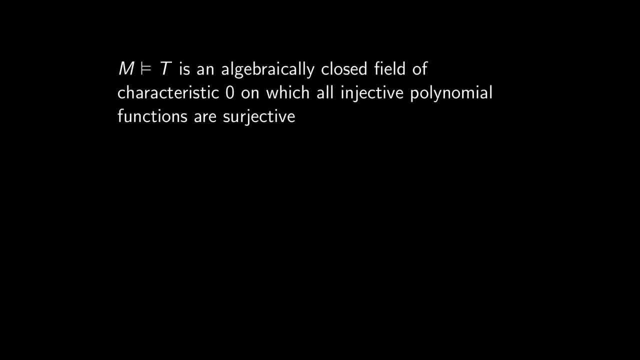 Let's look a bit more at this model. Well, it's an algebraically closed field of characteristic 0 on which all injective polynomial functions are surjective. But I don't really care that such a field exists, right? I wanted to study polynomial function in C. 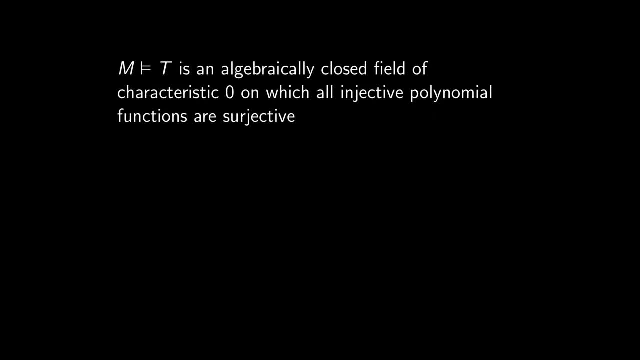 not in some weird abstractly-granted-to-exist field. Thankfully there is a very famous result of model theory, although famous here doesn't mean much because model theory in itself is not really famous. but a very famous result says: ACF is complete. 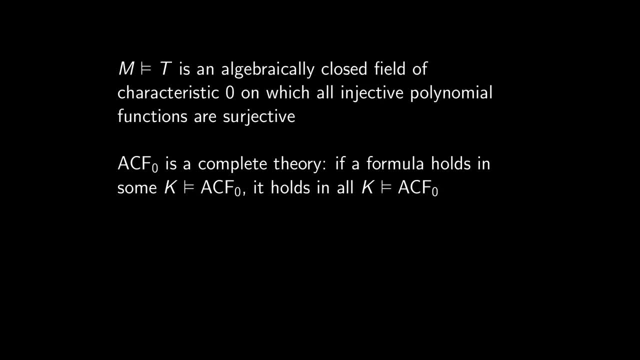 If a first-order formula holds in some algebraically closed field of characteristic 0, then it holds in all algebraically closed fields of characteristic 0. So all these shenanigans of injective-subjective functions, since it is first-order. 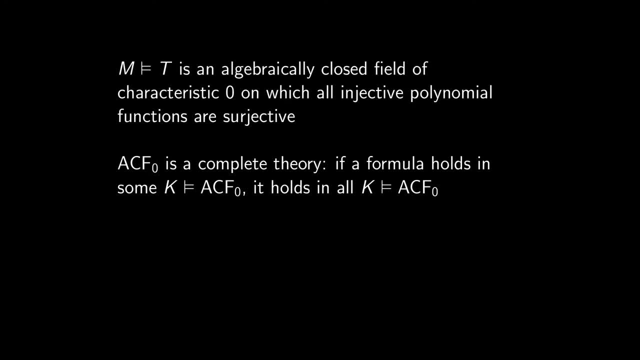 it holds in this model M that we just found. well, it holds in C. How amazing is that? We just proved that any injective polynomial function from C to the n, to itself is also surjective, and we didn't even have to do any fancy, complex analysis to prove it.